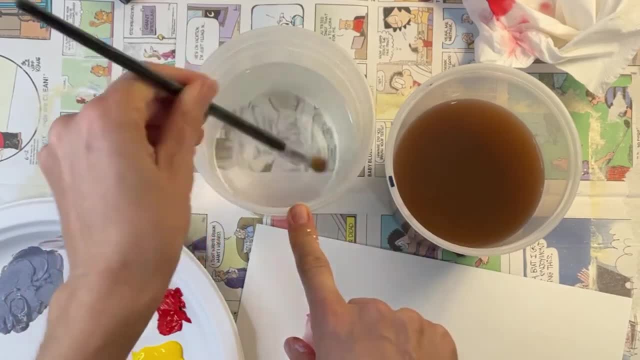 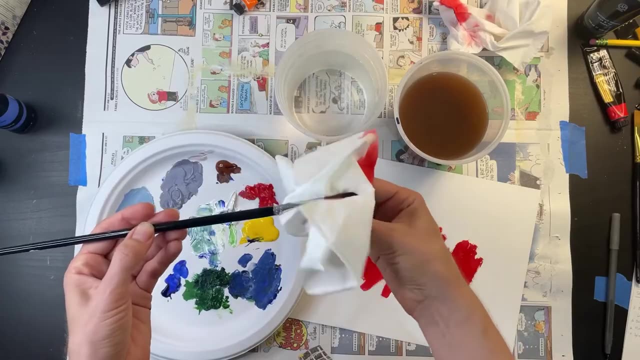 another water for your second rinse, And this water generally stays pretty clean. Okay, Now, before you go and get more paint, look how wet my brush is. You want to give it a pinch and windshield wiper in that tissue? Okay, So now I can start doing some yellow paint. 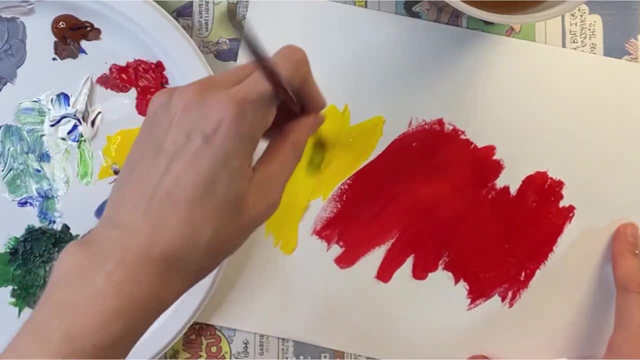 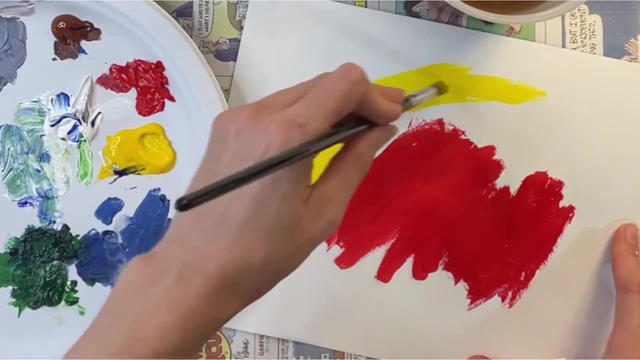 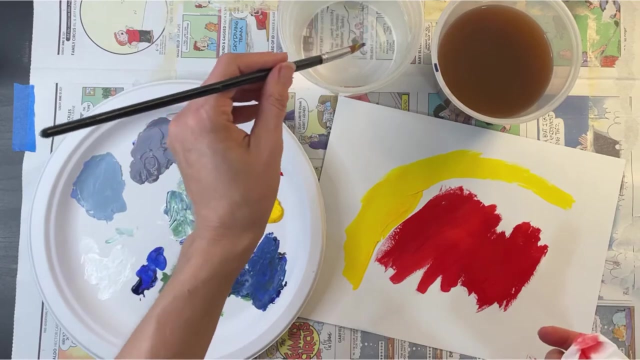 on here And let's say, I wanted to get like a really sharp line with my brush And I was having a hard time doing it. It was getting a little bit dry and scratchy. So what I can do is I can just dip my brush in the water like that and then continue painting, and then I'll be able to get a. 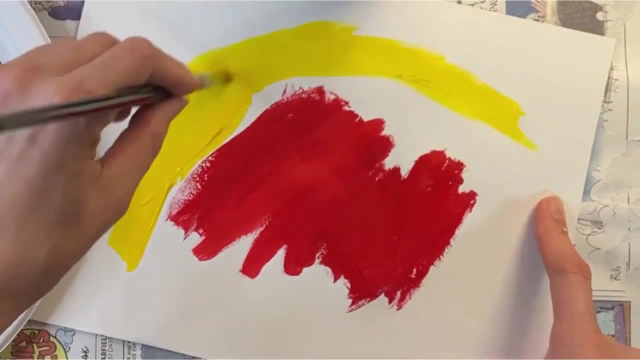 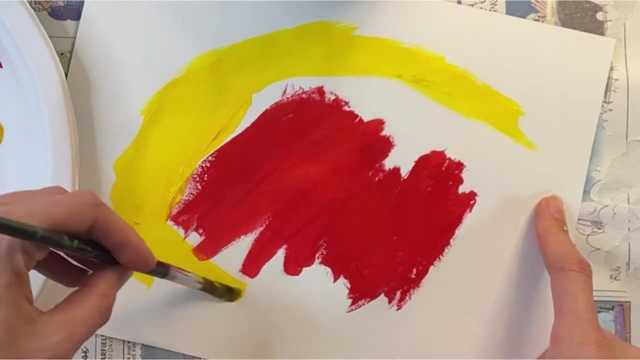 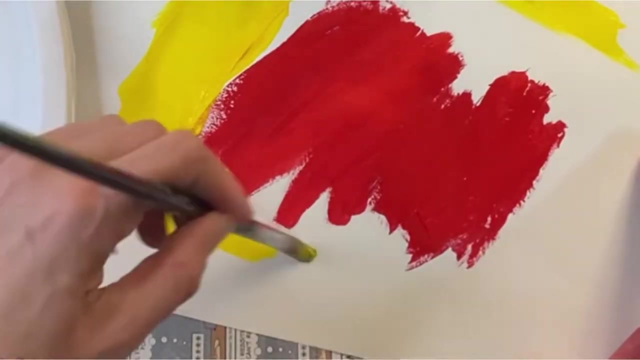 nice smooth line, okay. so that's a great tip for when, when you're painting and you're trying to get in there in these little detailed areas and, um, your, your paint's a little dry and scratchy, just dip it in the water like that and then keep painting and then you'll get really smooth nice. 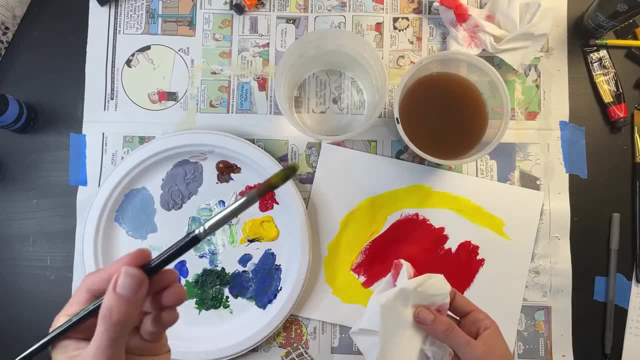 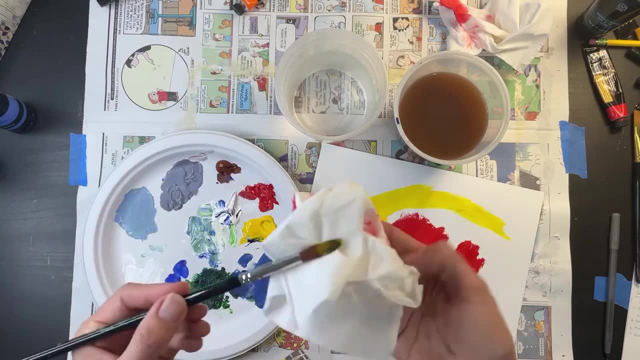 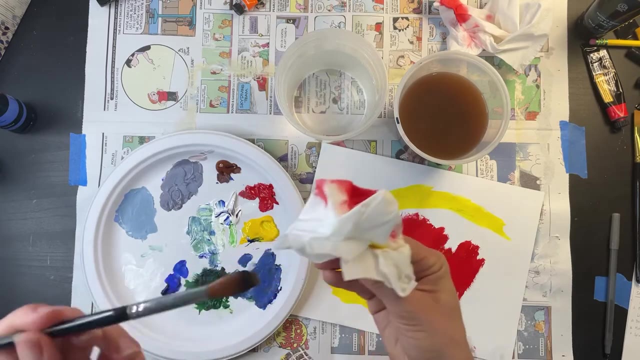 lines. okay. so one more time I'm going to remind you. so I have my yellow paint on my brush and I want to switch and get some brown now. so before I just go and get that brown, I'm gonna pinch windshield wiper, dip, pinch windshield wiper, and you got to make sure you end on that pinch. 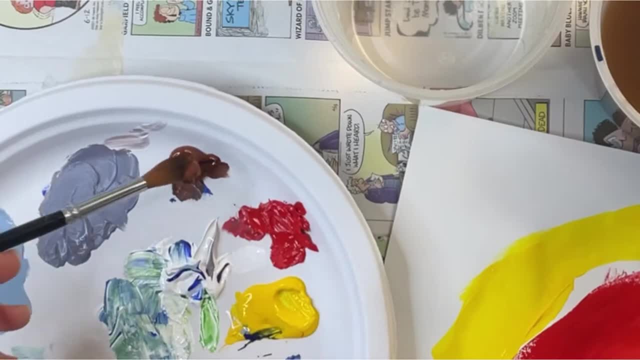 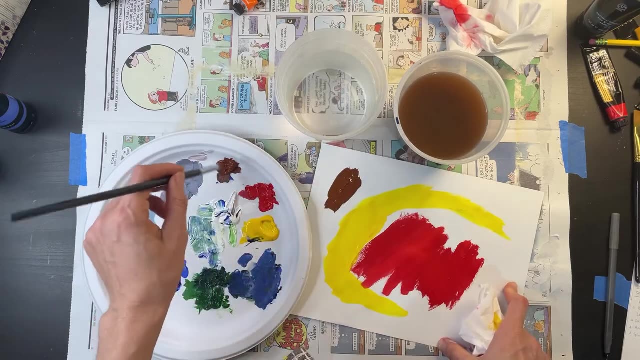 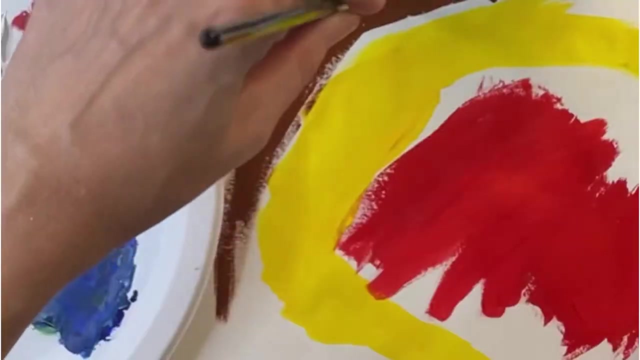 and windshield wiper so your brush is nice and dry when you go to get more paint. okay, because if your brush is super wet when you go to get paint, you're just going to get a bunch of water puddles in your in your paint. so this brown is pretty dry. see how dry this brown is. now you can. 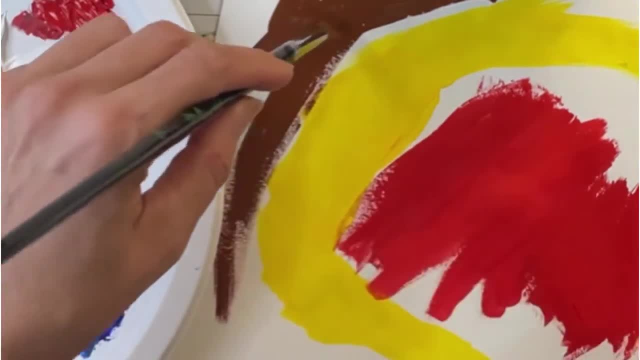 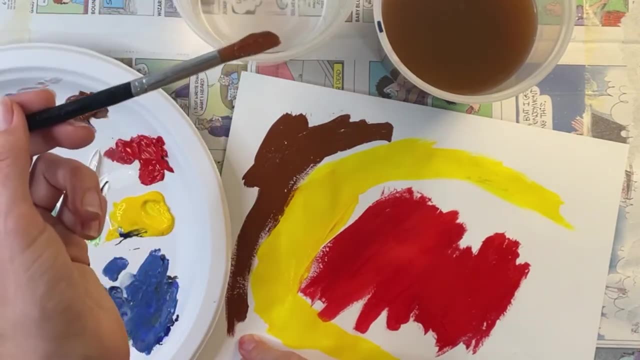 tell it's dry, because look at those little kind of scratchy scratchy marks there. so what i can do is i can just gently dip my paint in the water. don't stir it, just dip so you get a little water on your brush and then keep painting and you'll be able to do nice, smooth lines. if you found these, 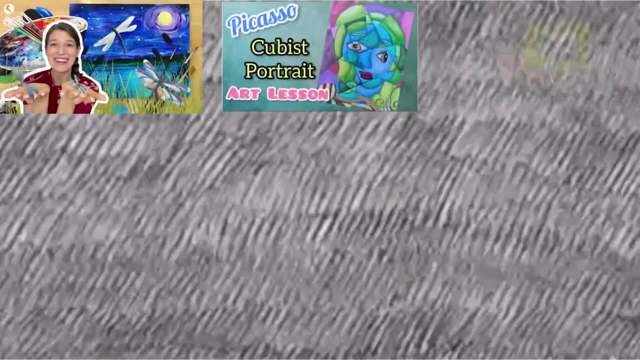 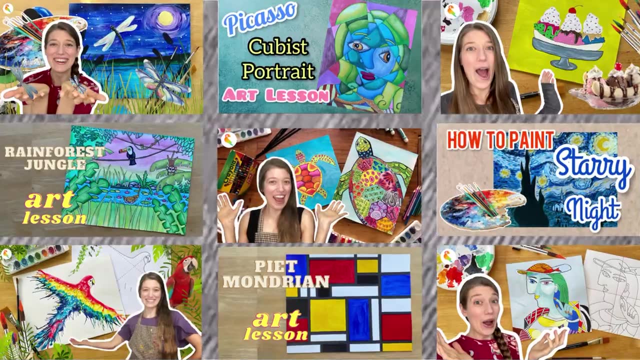 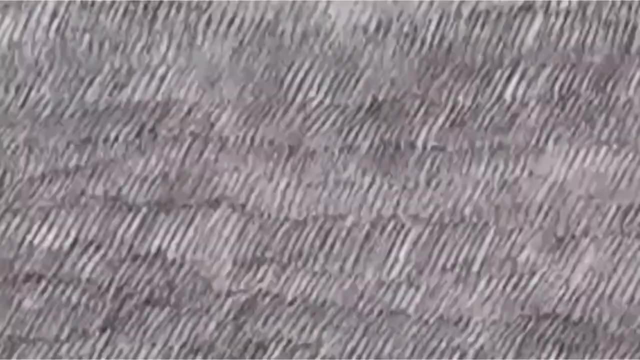 tips helpful. please hit that like button and be sure to check out the amazing art tutorials and step-by-step art lessons on my channel, rainbow parrot art.